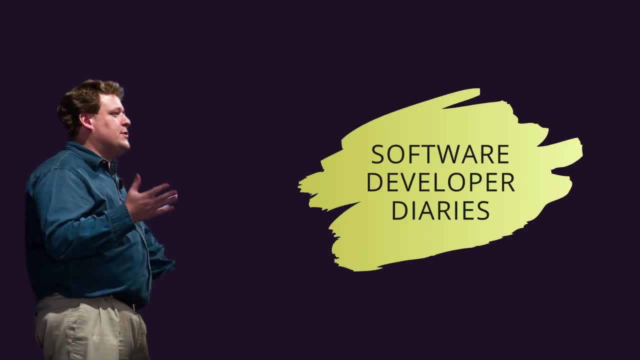 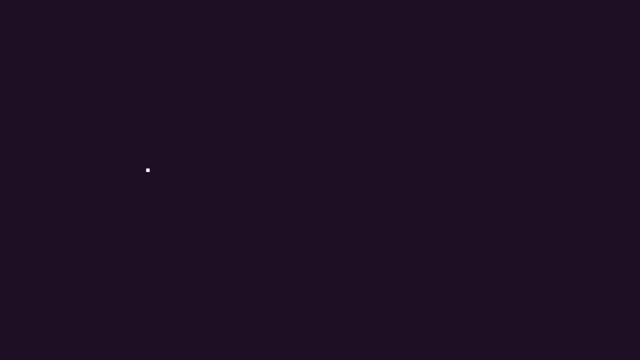 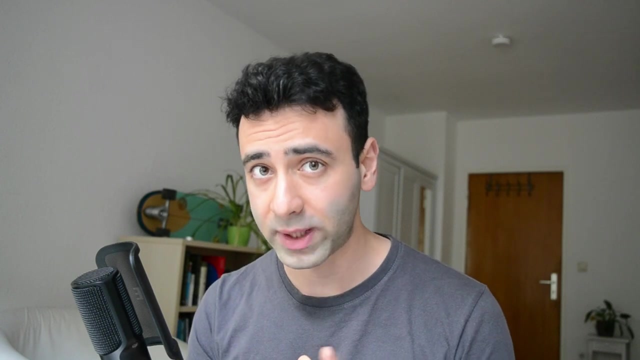 In 2000,, Roy Fielding proposed REST as an architectural approach to designing web services. Since then, REST APIs became the standard, but designing a REST API is still a challenge that many developers and teams tackle, even nowadays. It's very important to design REST APIs properly. 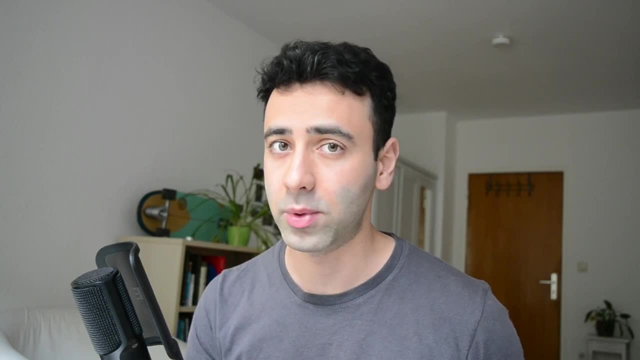 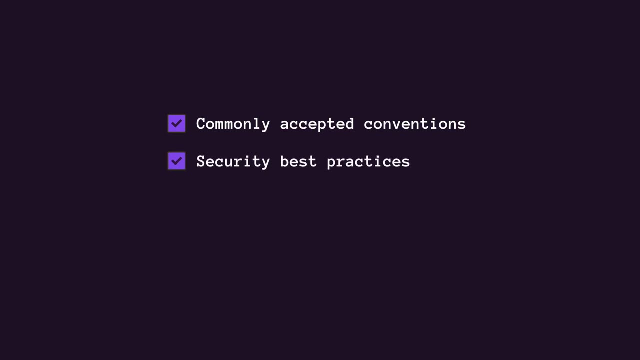 beforehand, so that we don't run into architectural problems down the road that can affect the whole infrastructure. We also take into account commonly accepted conventions, security, performance and ease of use for API consumers, And this is exactly what we're going to be diving. 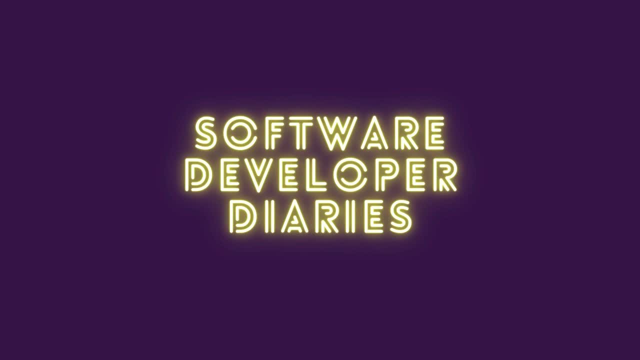 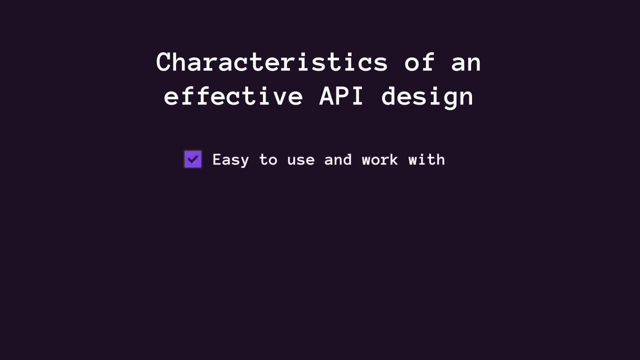 into in this video. In general, I would summarize an effective API design with three common characteristics: An API that is easy to read and work with, hard to misuse and which is complete and concise. By taking into account the points above, first we're going to look at one of the 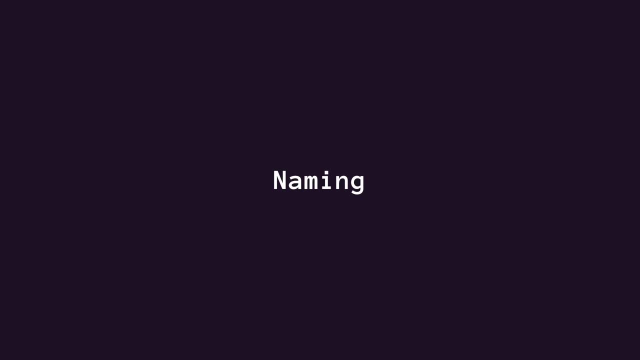 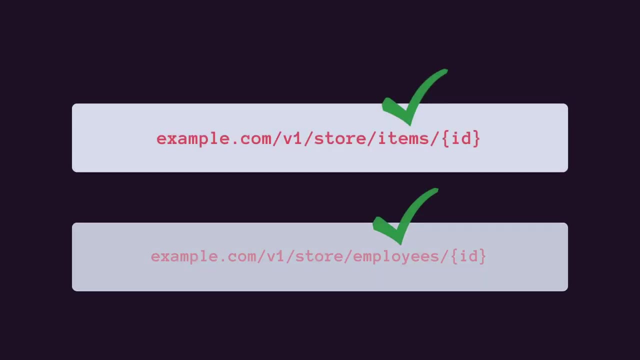 important aspects of the API design, which is naming. When defining an API endpoint, always make sure that the API design is well-defined. When defining an API endpoint, always make sure to use nouns to represent resources, not verbs. So in this example, we're going to use 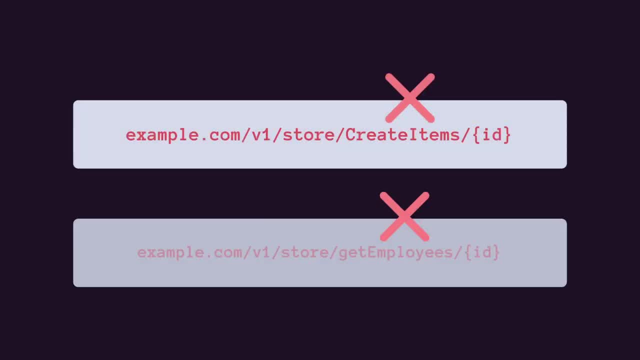 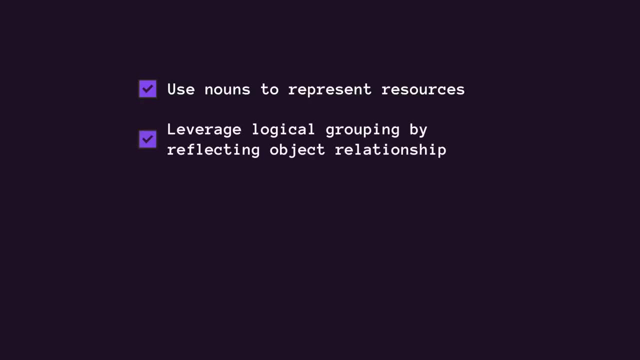 items and employees instead of create items or, for example, get employees. Also, when designing endpoints, it makes sense to leverage logical grouping, That is, if one object can contain another object, you should design the endpoint to reflect that. It's good practice, regardless of whether your data is structured like this in the database. 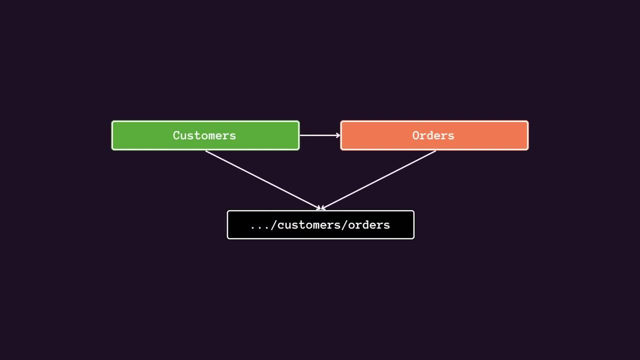 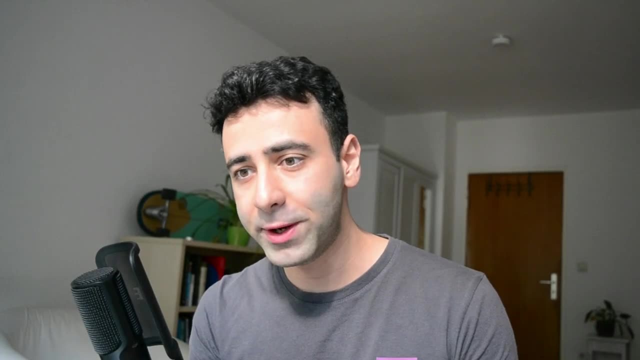 For example, if we want an endpoint to get the orders for a customer, we should append slash orders path to the end of the slash customers path. Also, I would advise avoiding reflecting the database structure with your APIs to avoid giving unnecessary information to attackers. 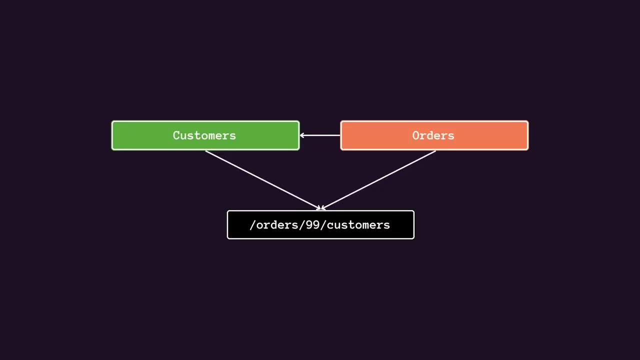 You could also go in the other direction and represent the endpoint from the order back to a customer with a URL such as orders slash, for example, 99 slash customer. However, extending this model too far can become cumbersome to implement. A better solution is to provide: 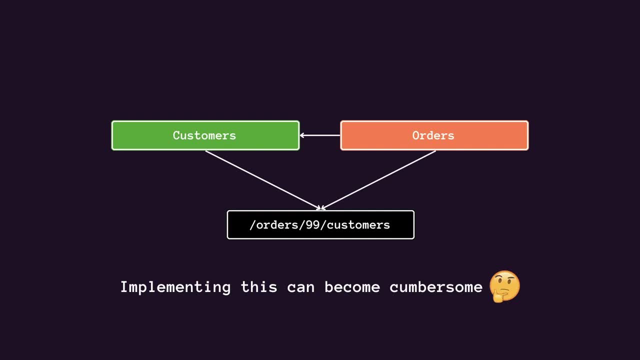 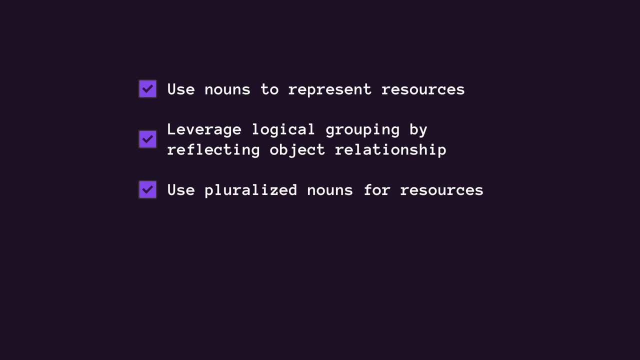 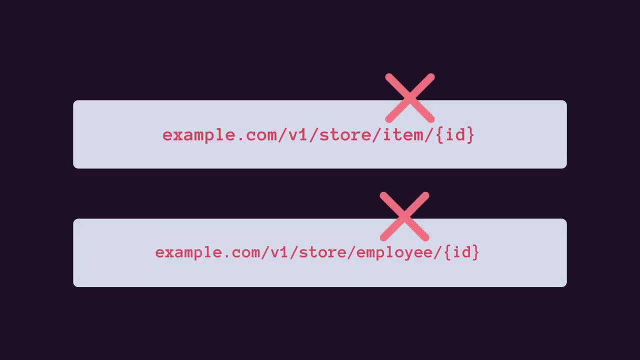 navigable links to associated resources. One possible solution is using hate OAS, which we're going to be looking into in a minute. Besides, when defining the names for your endpoints, use pluralized nouns for resources like items and employees, instead of item or employee. A resource has data and relationships. 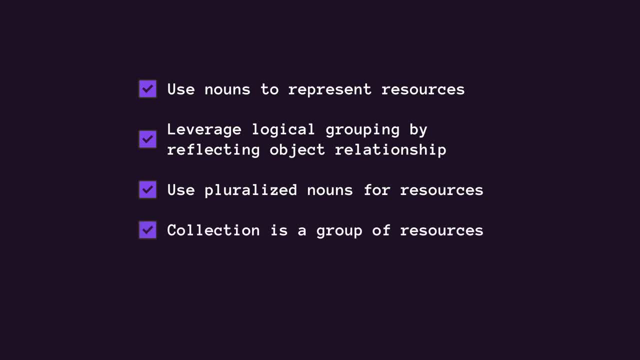 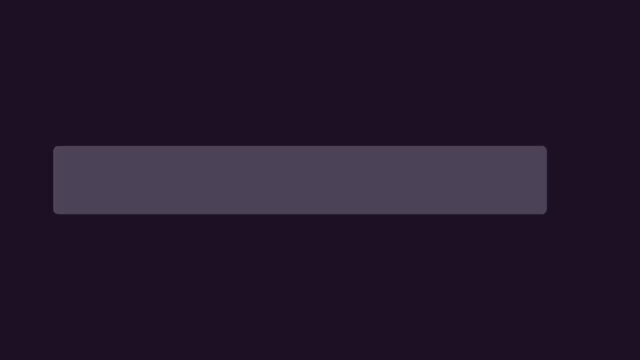 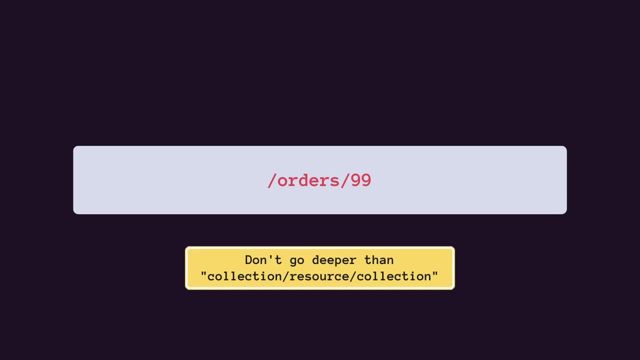 to other resources. A group of resources is called a collection. Just keep that in mind. For example, slash orders is a collection of orders Right And slash orders- slash 99 is a resource with information about a specific order. One important tip, though: try to avoid having complex URLs than collection. 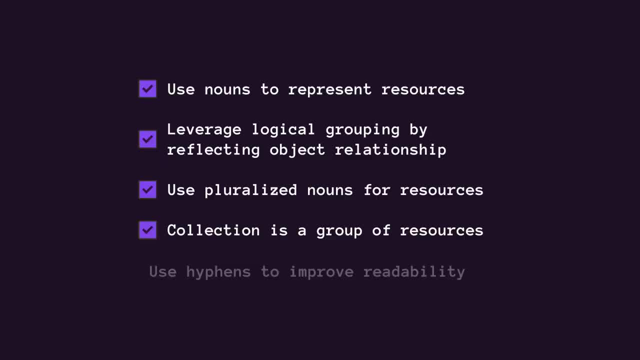 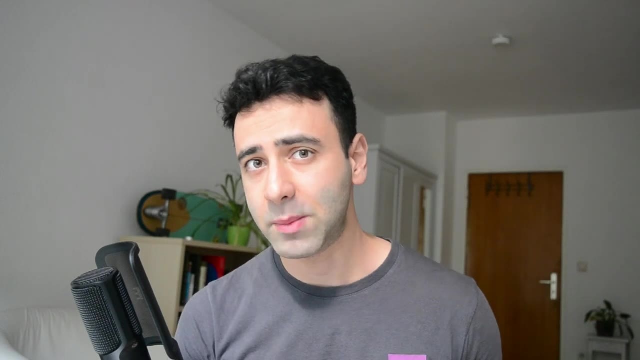 resource, then collection. Don't go deeper than that. Also, as a general rule, use hyphens to improve the readability of URLs, For example, inventory hyphen management instead of the underscore. Also, don't forget to properly version your API, Why? Well, imagine, thousands of customers are. 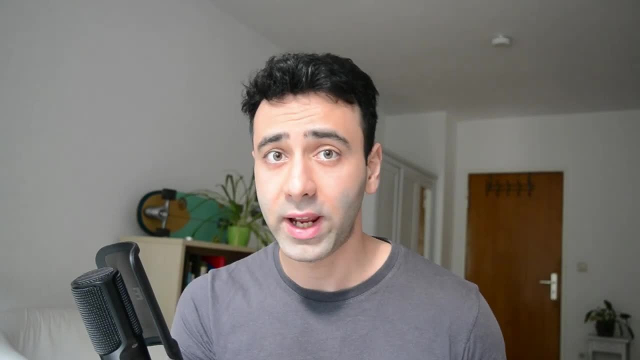 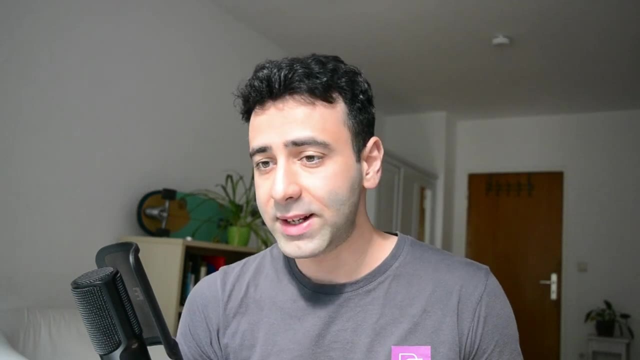 already using your API, but they don't know how to use it. If they don't know how to use it, they're already using your API and their applications are relying on it. What if you change one little detail in the URL name or in the response? Well then, all of these thousands. 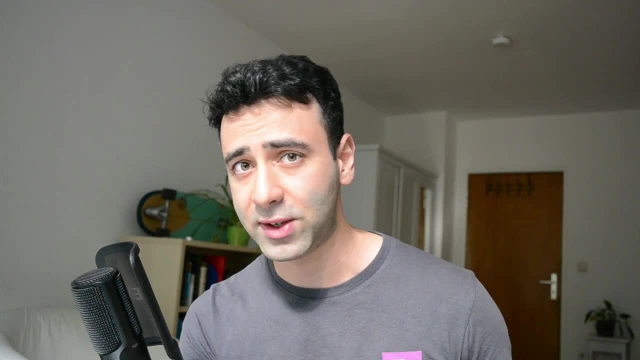 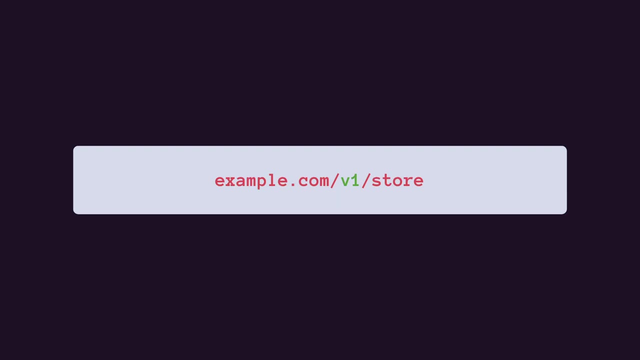 of applications are going to start breaking. This is not good. Luckily, you can always easily add a version path to your endpoints, For example, v1, slash store and so on. Alternatively, rather than providing multiple versions of URL, you can specify the version of. 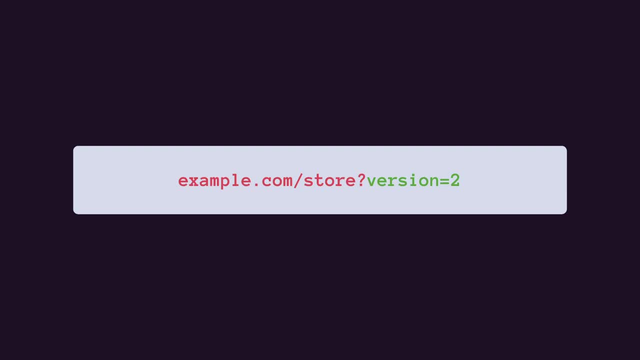 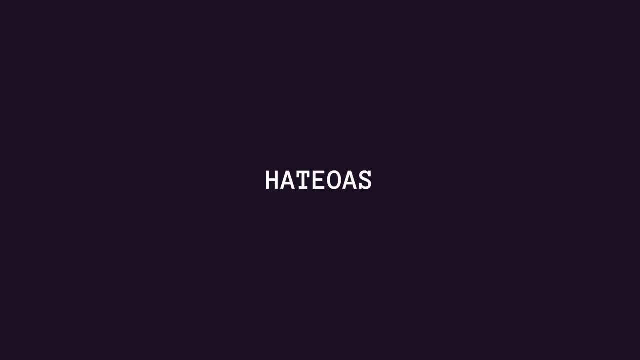 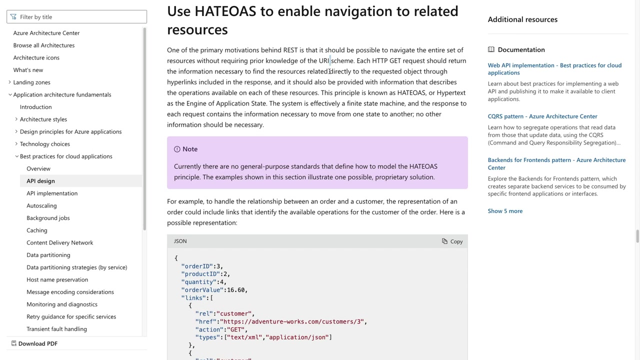 the resource by using a parameter within the query string appended to the HTTP request. For example, version equals two. In the previous point we mentioned hate OAS. Hate OAS makes it possible to navigate all resources without prior knowledge of the URI scheme. Each HTTP GET request returns. 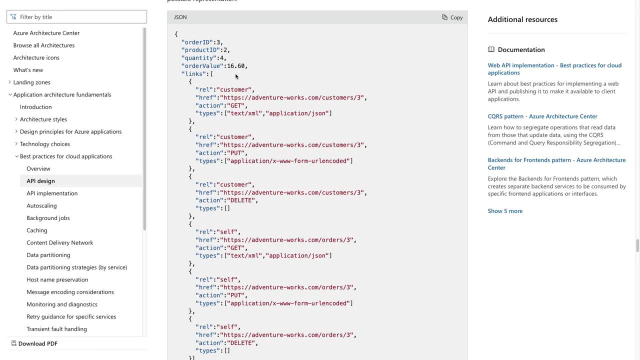 information to find resources related to the requested object through hyperlinks. The response also includes information that describes operations available on each resource, For example, to handle the relationship between an order and a customer. the representation of an order could include links that identify the available operations. 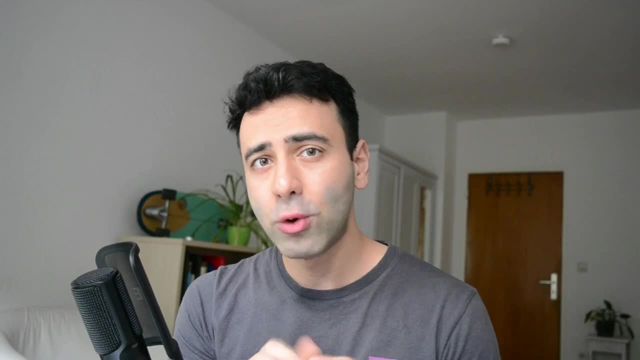 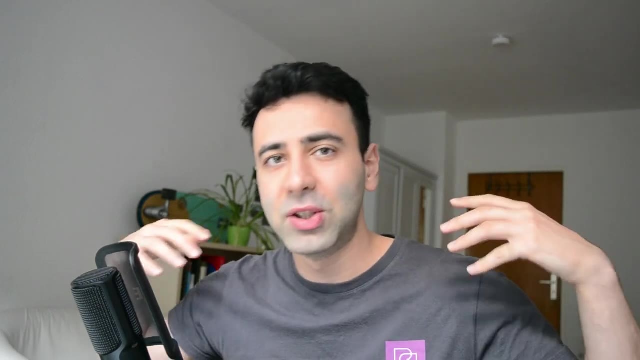 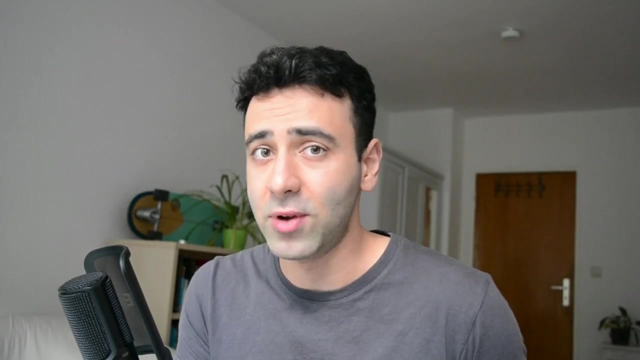 for the customer of the order. Currently there are no general-purpose standards that would define the proper usage of hate OAS. It's rather just there and you wouldn't stumble upon it very often, So it's just good to know that this thing exists in case if you ever need it in the future. 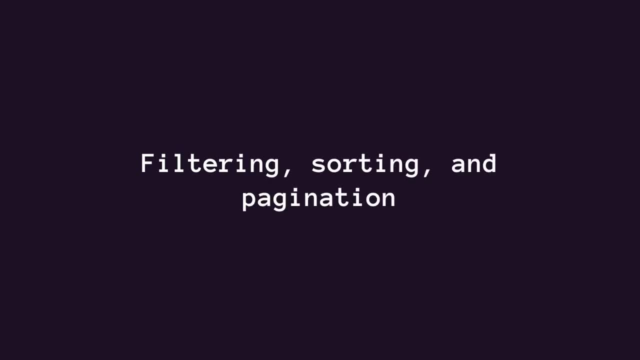 Our next point is the following. This point is crucial to have in every API. The databases behind the REST APIs can get very large, so we shouldn't assume that we're able to return all of that information in one go. Therefore, we need ways to filter items by supplying query parameters with specific key. 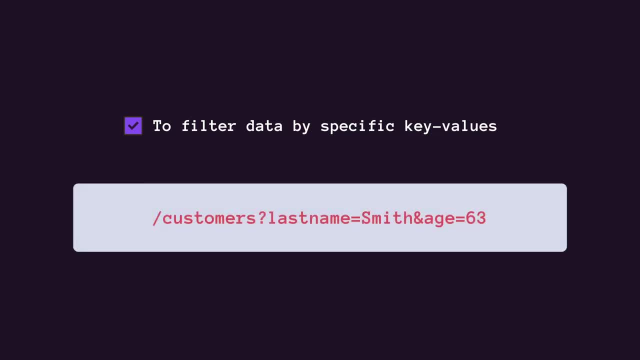 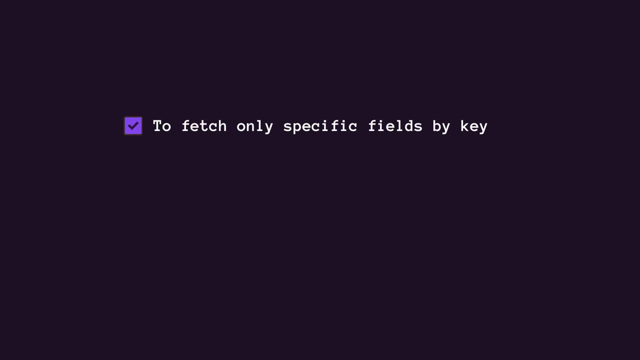 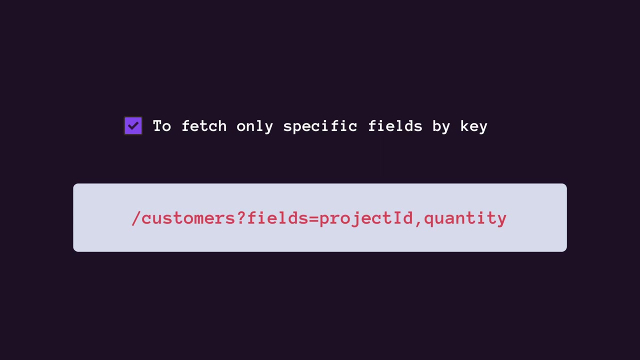 value pairs like lastName value and ageValue. You can extend this approach to limit the fields returned for each item if each item contains a large amount of data, similar to how you would want to fetch all columns of the database. For example, you could use a query string parameter. 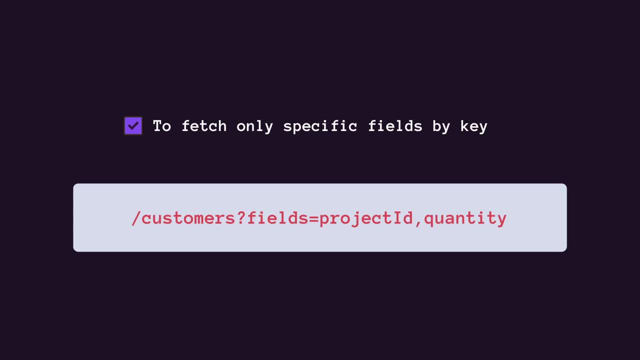 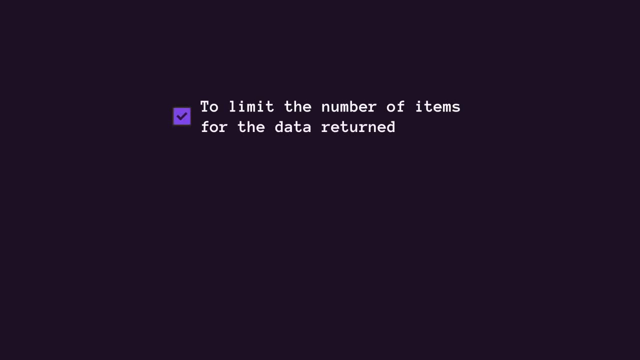 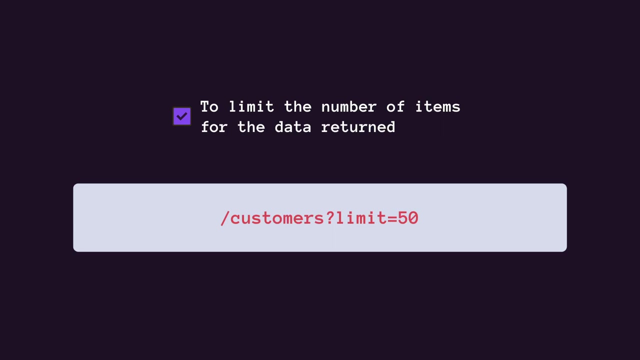 that accepts a comma-delimited list of fields such as productId or quantity. Obviously, we also want to have a way to paginate our data, meaning request specific chunks at one time, not to bring our database or services down by requesting all the data. Meaning 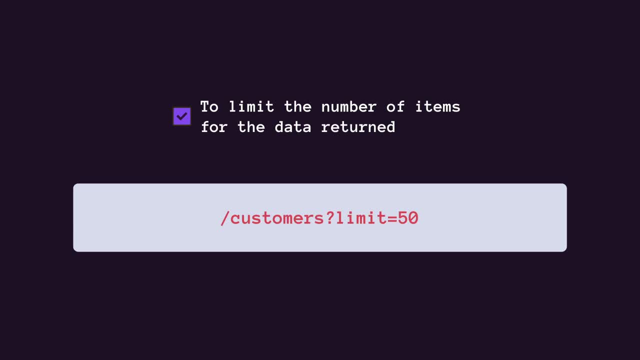 we can accept the limit query parameter and return a number of results that was specified. In order to paginate the results, meaning receive the next chunk, the user will have to supply an updated value for the start alongside the limit. Filtering and pagination obviously increase the performance of our queries, so 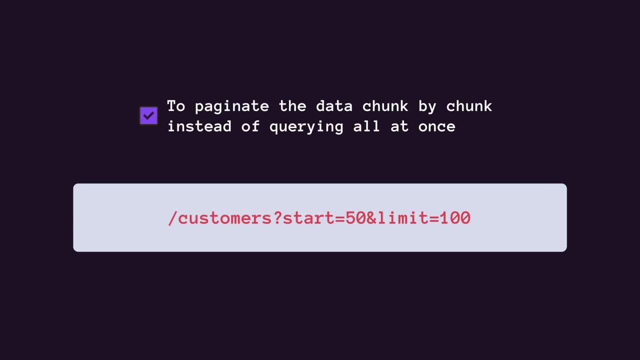 it's always good to keep those in mind. Additionally, we can also allow specifying the fields to sort by in query strings. For instance, we can get the parameter from a query string with the fields that we want to sort the data for. Then we can sort them by. 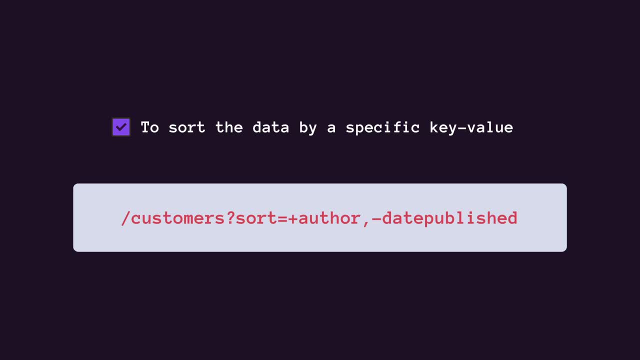 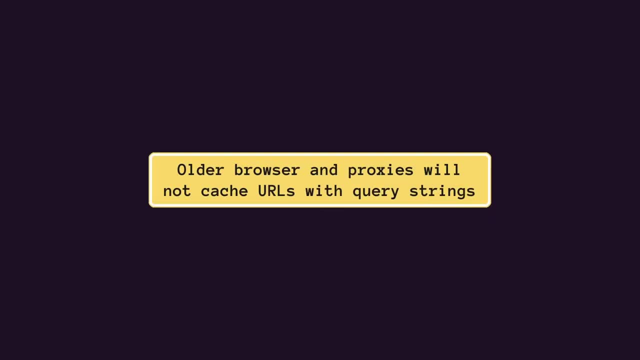 those individual fields, for example, plus author or minus date published. Keep in mind that some older web browsers and web proxies will not catch responses for requests that include a query string in the URI. One important rule that many developers miss is idempotency. 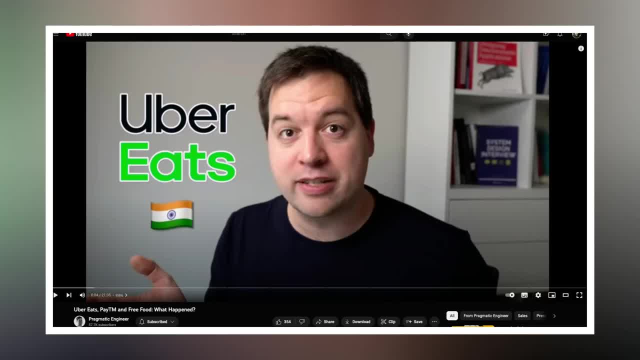 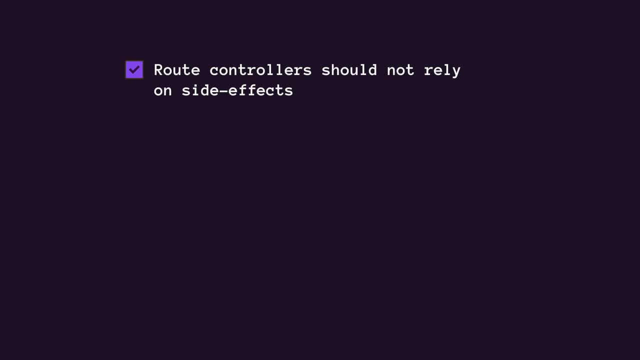 There's an interesting video covering the case of Uber Eats and how the customers were able to order pretty much unlimited food by making one of the endpoints non-idempotent. The code that implements the route controllers should not impose any side effect. The same request, repeated over the same resource, should result in the same state. 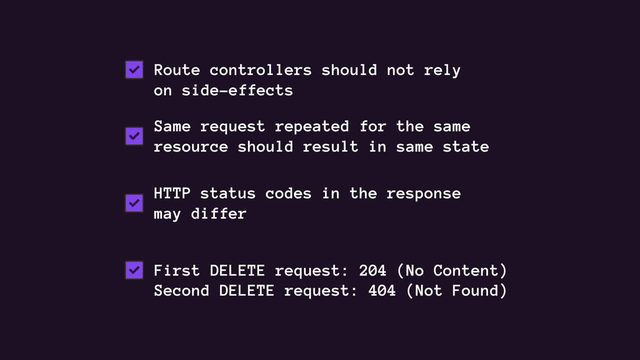 For example, sending multiple delete requests to the same URL should have the same effect, Although the HTTP status code in response messages may be different. That's totally normal. The first delete request might return status code 204, no content, while a subsequent delete request might return. 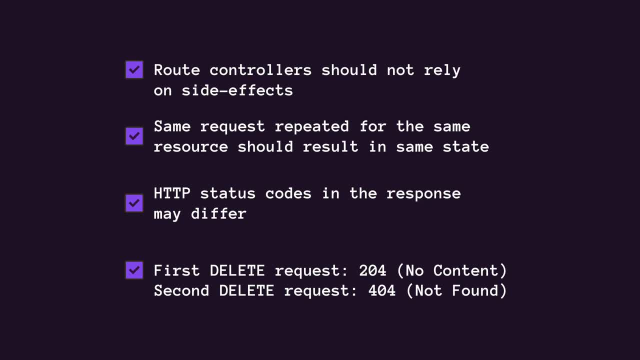 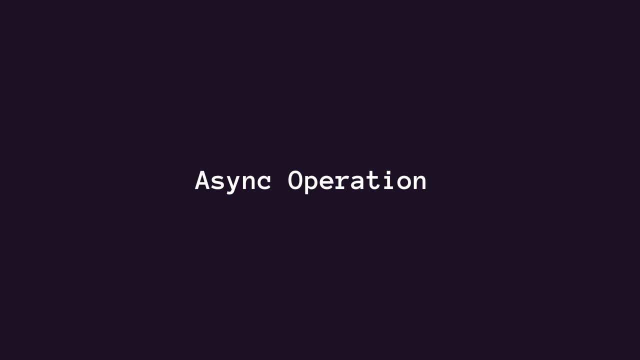 status code 404.. But the processing logic should stay idempotent. As a tip, make sure your controller methods are pure functions. Let's talk about async operations. Sometimes a post put, patch or delete operation might require processing that takes a while to complete. 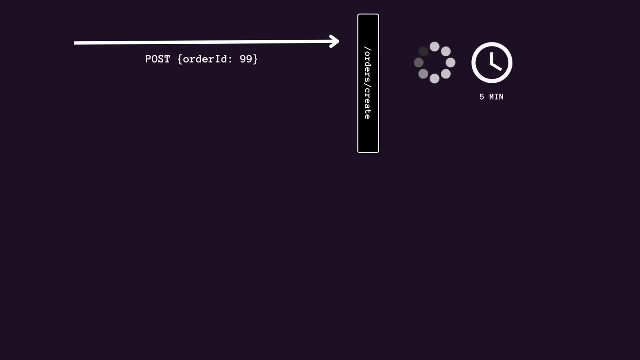 If you wait for completion before sending a response to the client, it might cause unacceptable latency. If so, simply consider making the operation asynchronous. Just return HTTP status- code 202, to indicate that the request was accepted for processing but not completed. You should also expose an endpoint that returns the status of the asynchronous request. 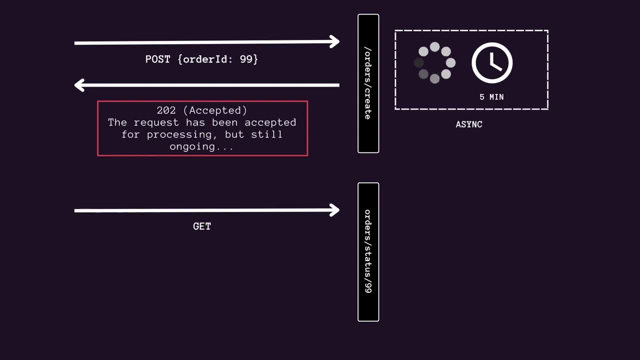 so the client can monitor the status by polling the status endpoint. Also include the URL of the status endpoint in the location header of the 202 response. If the client sends a GET request to this endpoint, the response should contain the current status of the request. 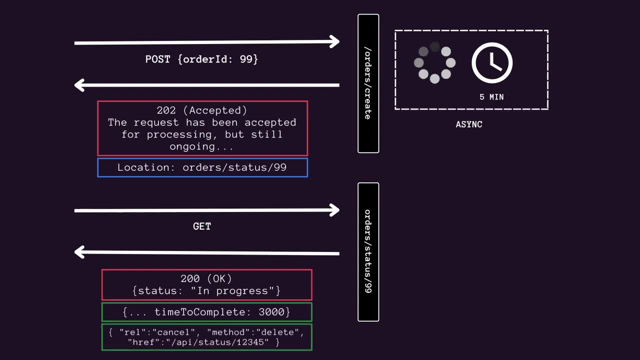 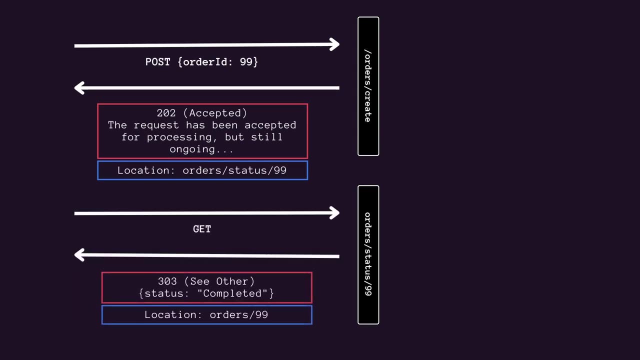 Optionally, it could also include an estimated time to completion. You should also include a link to cancel the operation. If the asynchronous operation creates a new resource, the status endpoint should also return the status code 303 after the operation completes. In the 303 response, include a location header that gives the URL of the new resource. 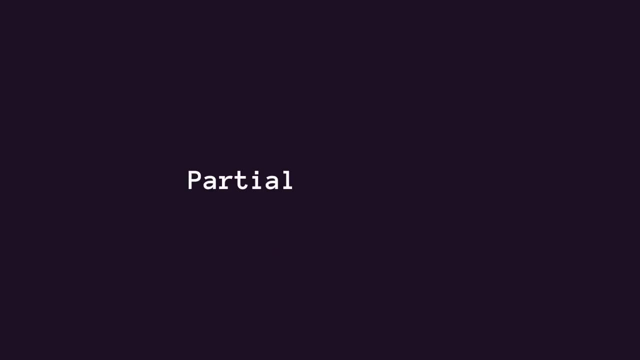 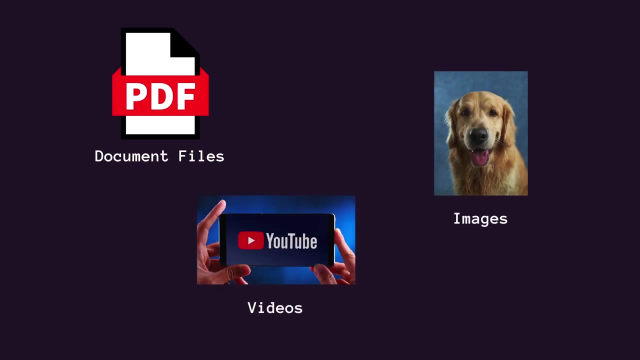 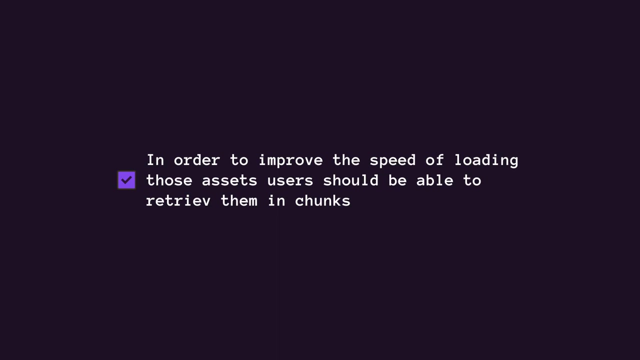 As the product gets more complex, a need for supporting partial responses in your REST API comes up. Large binary fields like files or images may be included in a resource. To improve response times and overcome issues with intermittent connections, we need to enable the retrieve of these resources in chunks. 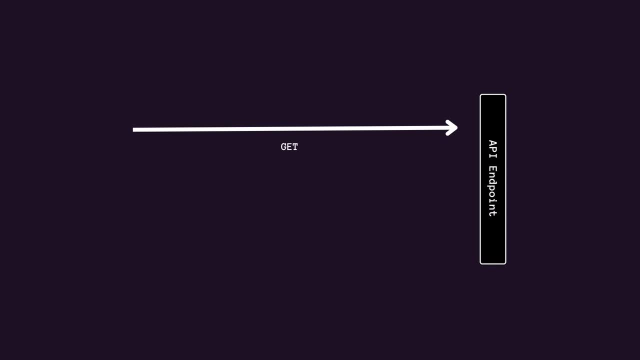 To do so, the API should support the AcceptRanges header for GET requests of large resources. This header allows partial requests for specific byte ranges of a resource which can be submitted by the client application. Also, consider implementing HTTP HEAD requests for those resources. 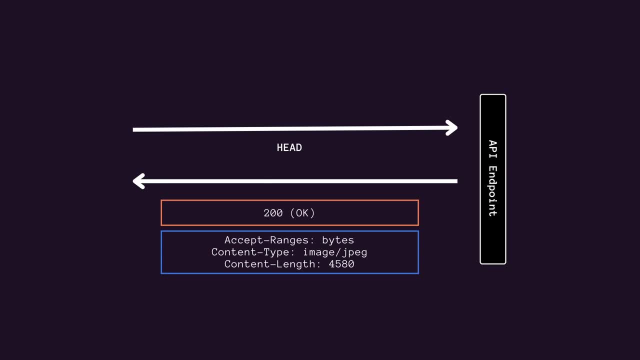 A HEAD request is similar to a GET request except that it only returns the HTTP headers that describe the resource. with an empty message body. A client application can issue a HEAD request to determine whether to fetch a resource by using partial GET requests. The ContentLength header here gives the total size of the resource. 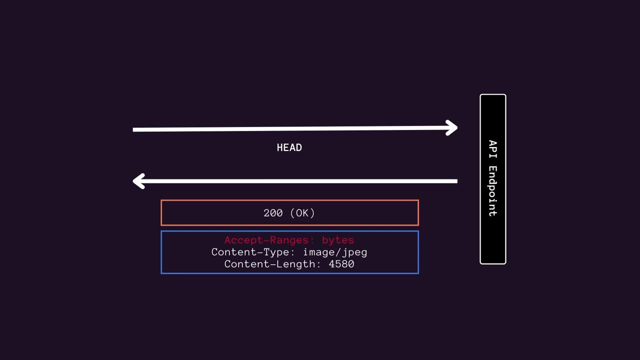 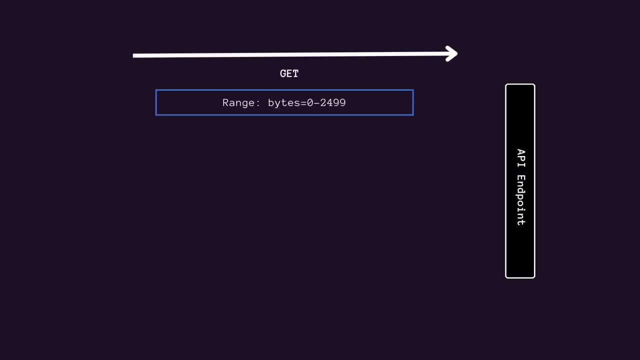 and the AcceptRanges header indicates that the corresponding GET operation supports partial content. The client application can use this information to retrieve the image in smaller chunks. Then the first request fetches the first 200 or 2500 bytes by using the Range header. 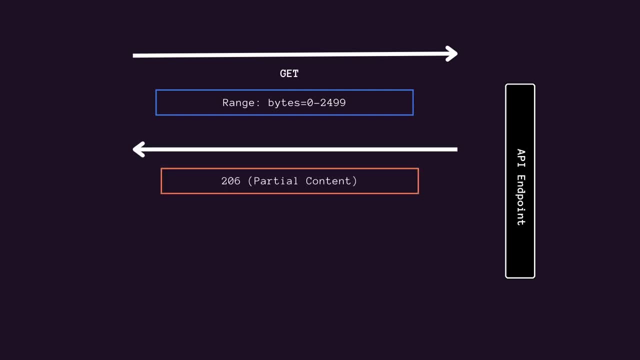 The response message indicates that this is a partial response by returning an HTTP status code 206.. The ContentLength header specifies the actual number of bytes returned in the message body And the ContentRange header indicates which part of the resource- this is A subsequent request from the client application can retrieve the remainder of the resource. 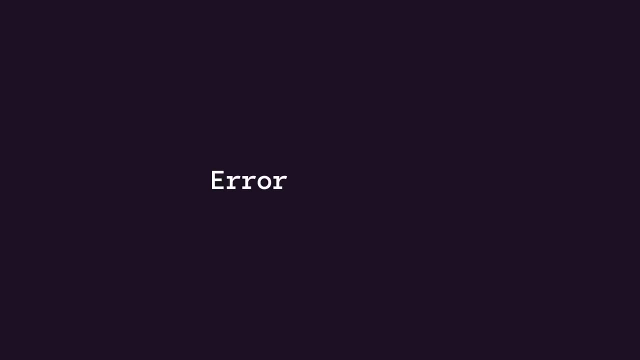 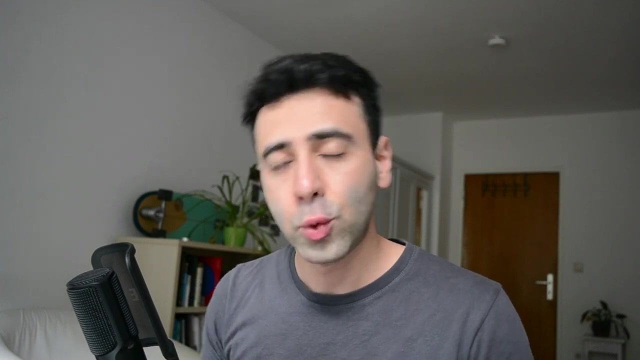 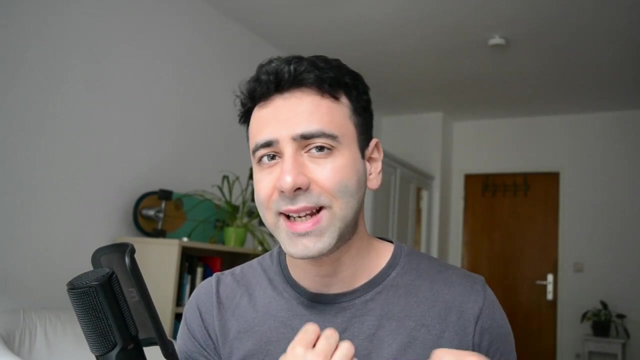 just very similarly to pagination Error handling. There's no way we can miss this one. To eliminate the confusion for API users whenever errors occur, we should gracefully handle these exceptions and return a proper error response code so that it kind of gives a clue to the developer how they can debug this issue. 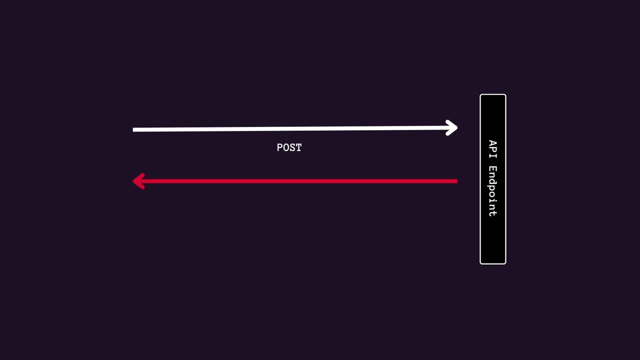 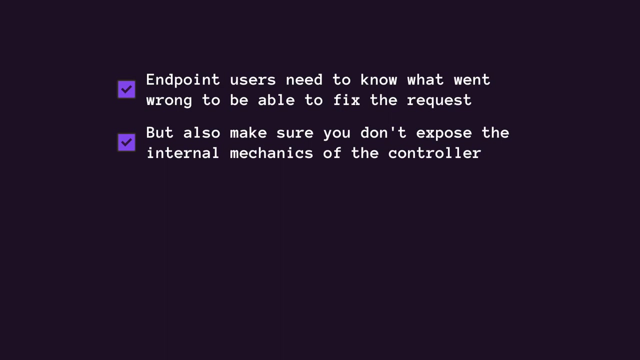 Error codes need to have messages accompanied with them so that the maintainers have enough information to troubleshoot the issue, but attackers cannot use the error content to carry out attacks like stealing information or bringing the system down. Be very precise with the codes that you return. 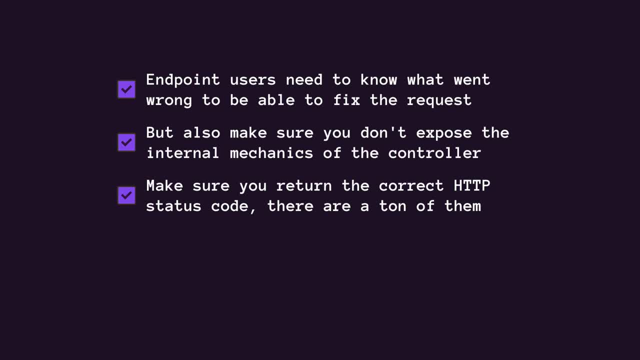 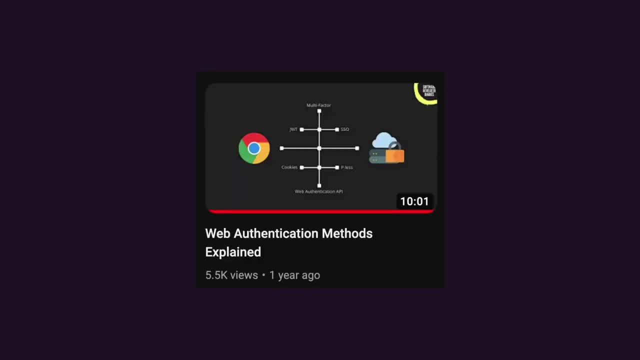 For example, any time the body of a successful response is empty, the status code should be 204.. Have you already watched my video on authentication? If not, I would highly suggest watching it first. But here are the basic milestones that every REST API should consider. 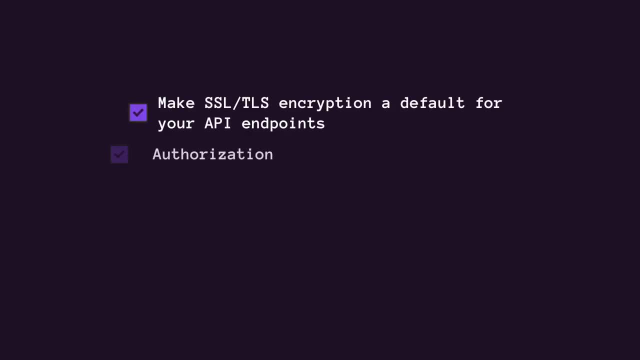 for the basic security, First of all, using SSL or TLS encryption. obviously Also, a normal user shouldn't be able to access information of another user. They also shouldn't be able to access data of admins. We're going to talk about the concept of ACLs in the future videos. 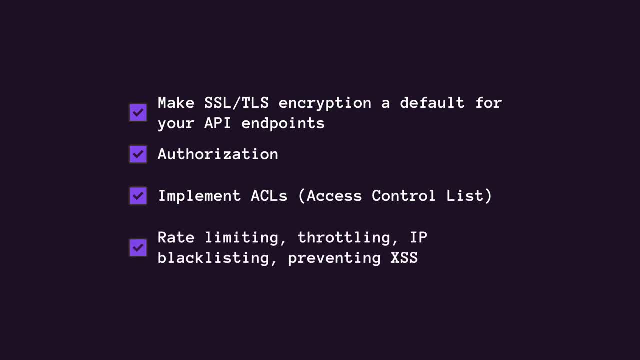 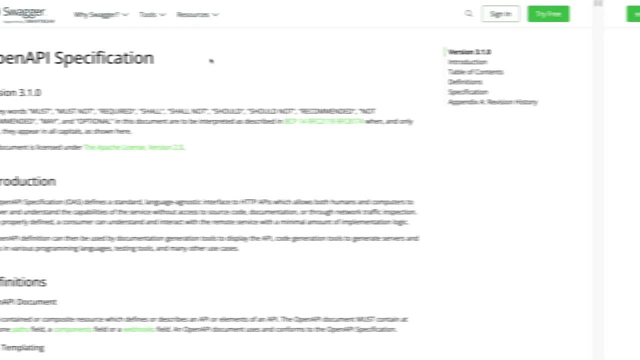 Also track clients and implement throttling to reduce the chances of DOS attacks. Last but not least, it's worth mentioning OpenAPI, formerly known as Swagger, which is an open-source API standard for describing, documenting and visualizing RESTful endpoints.